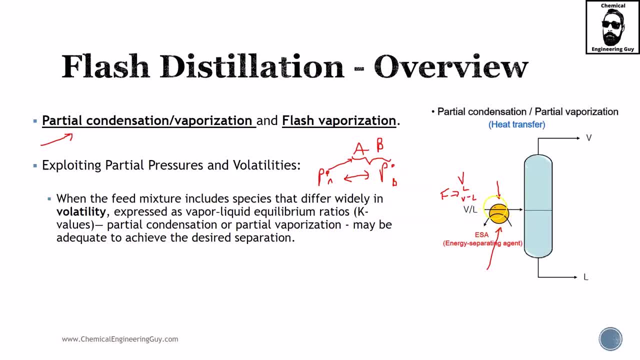 maybe you want to use a valve in order to change pressures or a heat exchanger in order to change temperatures. The main idea is, of course, that once the mixture is right here, it separates into vapor and liquid. Now, the interesting part right here is not that this is just a simple separation, Rather 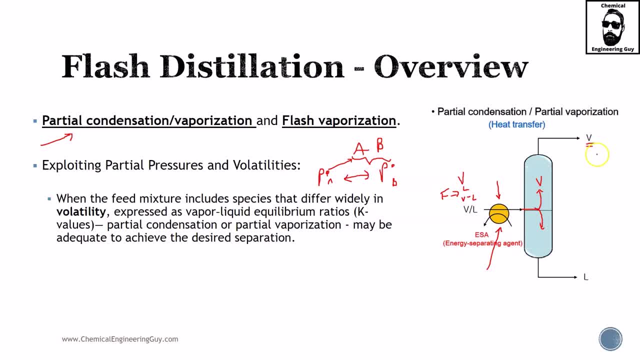 the vapor will be separated. So let's say that we have a rich in volatile material And let it be that A is the most volatile material- I will use a lot of MVC- meaning most volatile material- And B will be the least volatile. 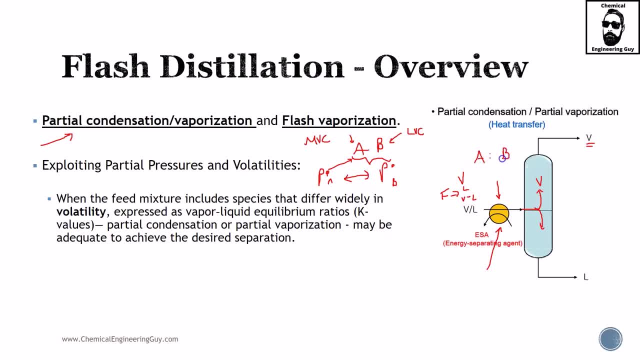 material. So let's say that we have A and B almost 50-50.. The main idea is that the component A will be richer in the vapor phase And, of course, component B, the least volatile material, will be richer in the bottoms. 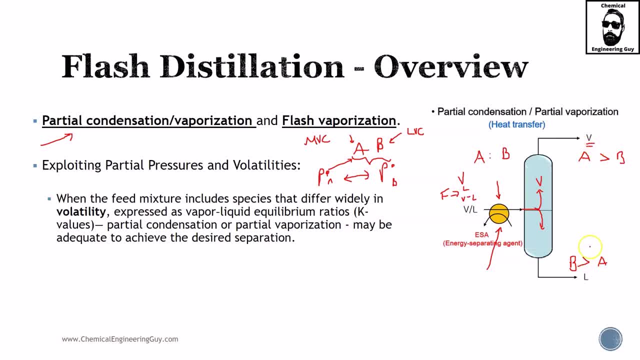 So typically you will hear destillates and bottoms or vapor and liquid streams or product and subproducts lines. okay, Overall, that's the idea: to separate and get richer A and richer B. Let's start reading a little bit more on this. 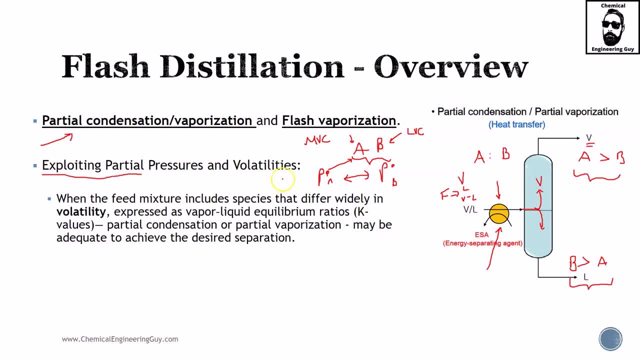 The main idea is, of course, stated before: exploit the partial pressure differences or the volatility differences between two components. Now, of course, if A and B are pretty similar in vapor pressure, it will be hard and probably you will get pretty similar streams right here. 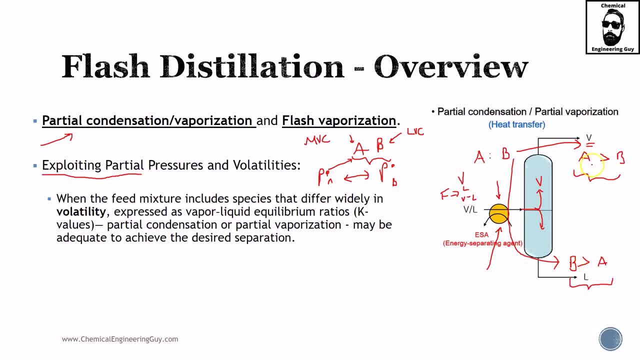 But if they are far away from each other, you will have what we already stated: A vapor with rich volatile material and a liquid with rich non-volatile material When the feed mixture includes species that differ widely in volatility, expressed as vapor-liquid equilibrium ratios. 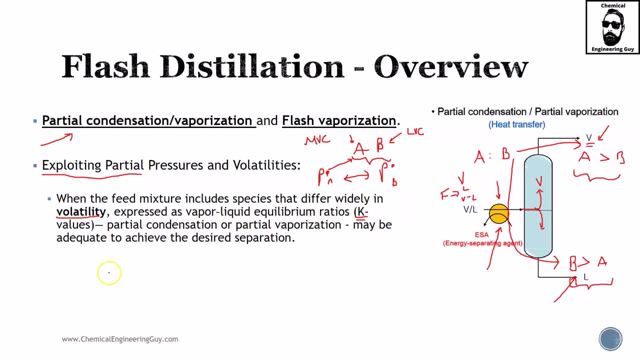 Remember, if you have been taking physical chemistry or maybe thermodynamics, you know this concept of k-values, which is nothing more than the composition, the vapor phase, versus the composition in the liquid phase of a species. let it be I, It can be methane, propane, octane and so on. 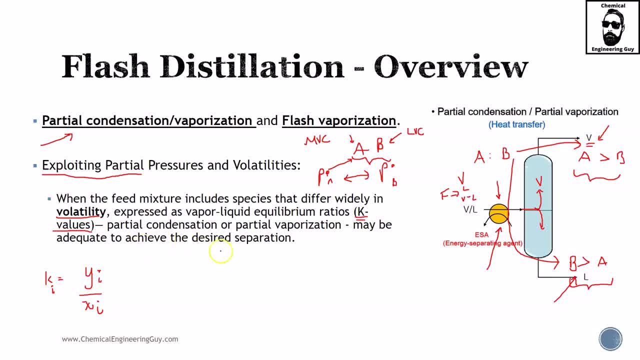 Partial condensation or partial vaporization may be adequate to achieve the desired separation. So, technically speaking, we are saying this partial condensation or partial vaporization may be adequate to achieve the desired separation, But the actual separation occurs when you send this mixture inside this drum. 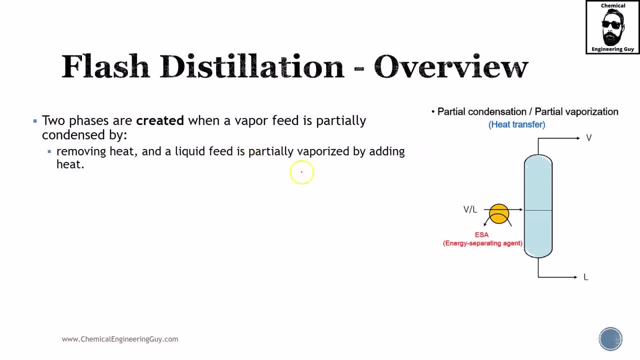 Two phases will be created when the vapor feed is partially condensed. So, as you can see in this example, we are having a feed which is partially pure vapor. Then you add a chiller and then you get a mixture of vapor-liquid. So the removal of this heat will force liquid formation, of course, because we are condensing. 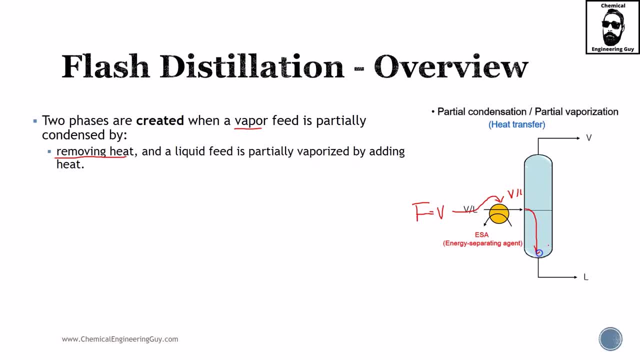 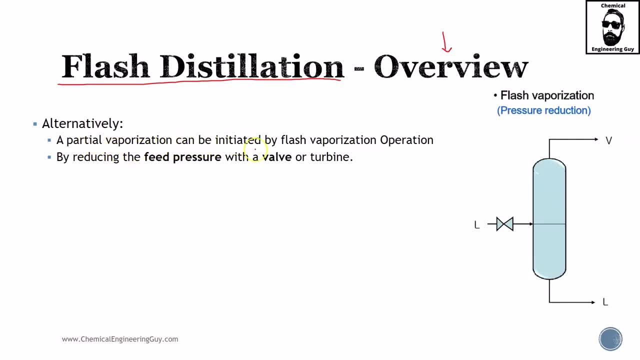 it. Of course, liquid falls down due to gravity, vapor goes upwards. Alternatively, a partial vaporization can be initiated by flash vaporization, by reducing feed pressure with a valve. So this is interesting. I stated before we can use either a chiller or heater, or you can use a valve or pressurizer. 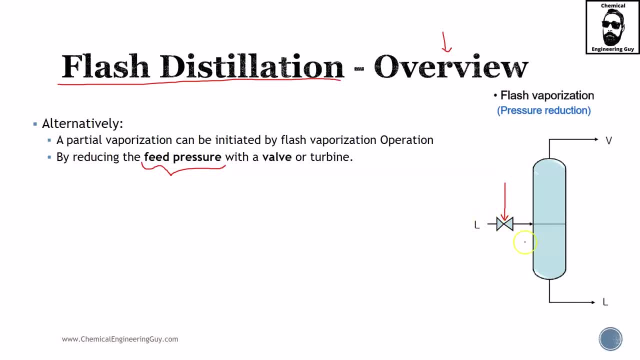 right here. Of course, if you're using a pressurizer, most likely you're going to be forming a liquid, And if you're using a valve, most likely you are producing air. So this is interesting. I've stated before we can use either a chiller or heater, or you can use a valve or pressurizer. 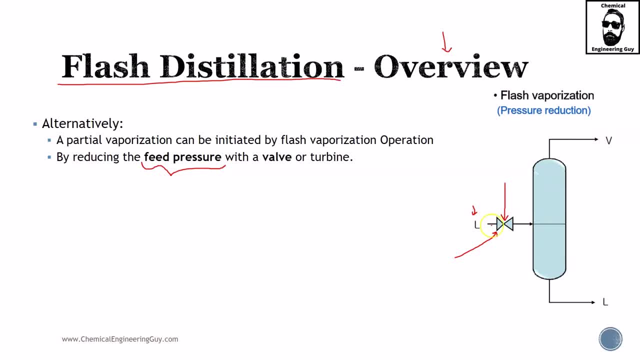 And if you're using a vapor, So if you have a liquid which is near its bubble point, then getting it full throttle in this valve, you will have vaporization, And what you want to do, of course, is vaporize upwards. the liquid fall down. 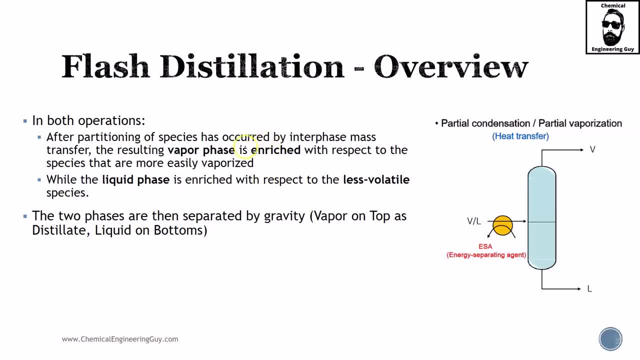 In both operations, after partitioning of species has occurred by interface mass transfer- We have been talking already about this- The resulting vapor phase is enriched. enriched meaning that the most volatile material will be of greater amount here, while the liquid phase is enriched with respect to the less volatile. 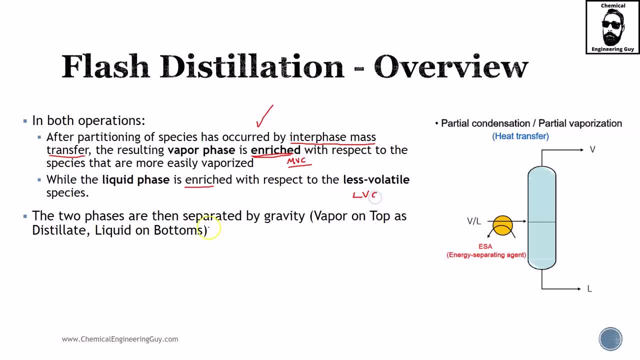 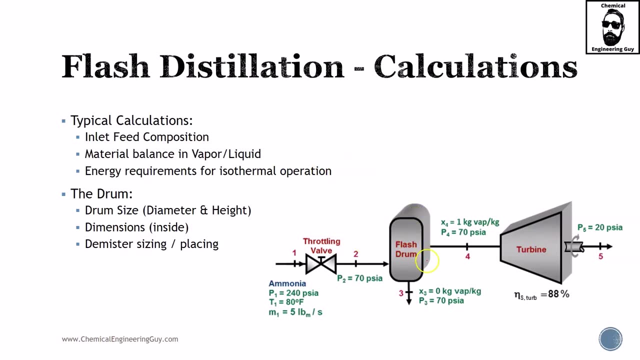 material, or i like to call it least volatile component. the two phases are then separated by gravity. so, as you can imagine, vapor goes upwards and liquid goes downwards. so let's talk about the calculations. what would you typically be doing whenever you are in charge of designing or operating a flash drum or controlling a flasher? so typical calculations. 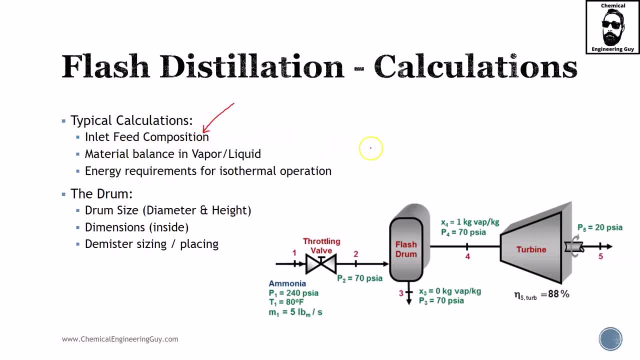 will be. what is the inlet feed composition? what are your vapor requirements, how much amount and how pure vapor you require, the bottoms, the equilibrium interactions overall, the material balances and also energy requirements. so, if you're talking about isothermal operation, or maybe you're talking about adiabatic operation, if you're going to be cooling it or heating it, if you're going to, 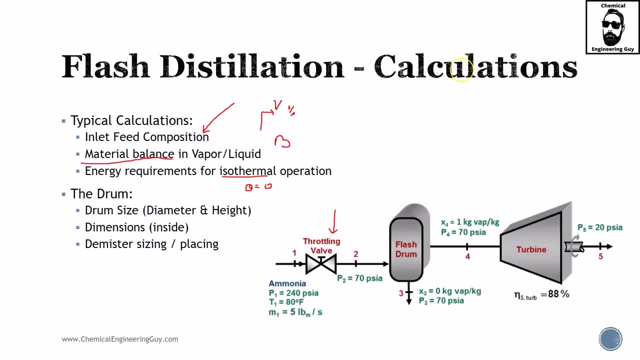 be changing pressure here or not? well, that's all the type of calculations you will be required. i'm probably wondering: what about the drum? well, you will need to flash, or let's say, size the flash drum, depending on how the diameter versus height should be the inside dimensions, which of 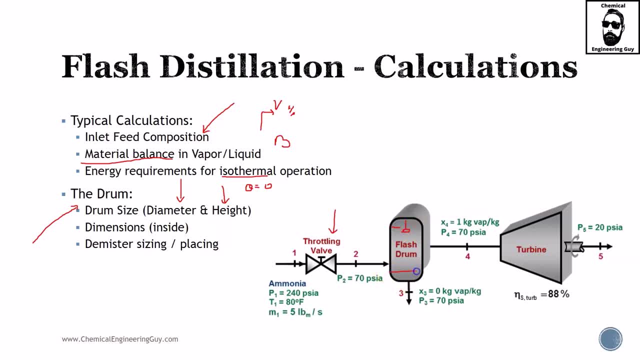 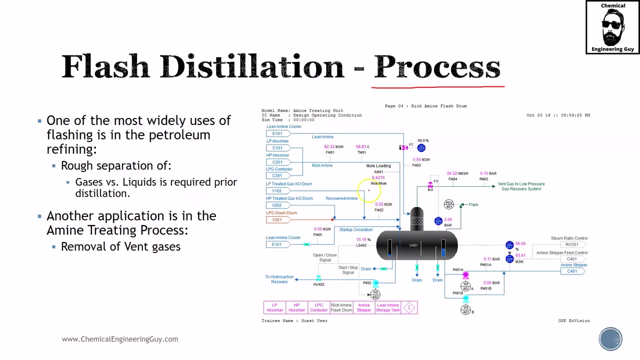 course, you will see that you need to add a mesh. and how heights? the nozzle inlet height, how the ratios of distances- well, heights, technically will be calculated here- and all the dimensions which, of course, will be more of a detailed design. and talking about the process, well, probably you have in mind some processes. flash distillations are very commonly used in the 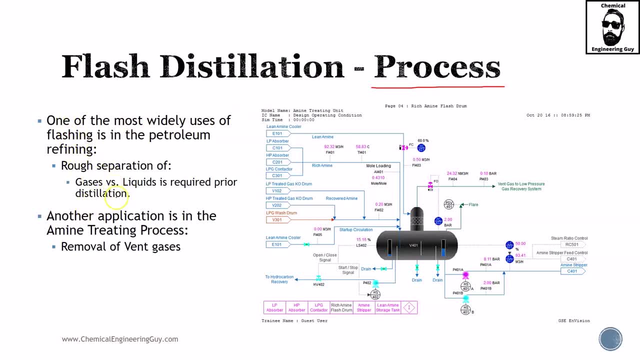 industry. right, i decided to use this one right here. so many applications in the petroleum refining will have, let's say, a lot of liquids which have some gases within which are very, very non-compressive, let's say they cannot be condensed. let it be methane, let it be hydrogen, and if you're talking, 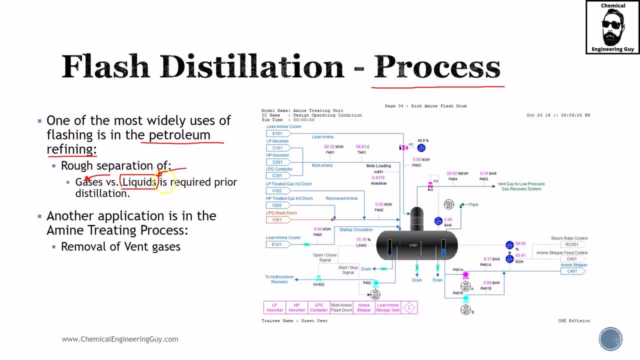 about more heavy materials such as gasoline. well, even though you may try to liquefy methane well, gasoline is already a liquid at the standard conditions. instead of bothering in condensing gases, what we do is use a flash drum and get rid of these gases. you can either send them to a vent or into another separation unit. 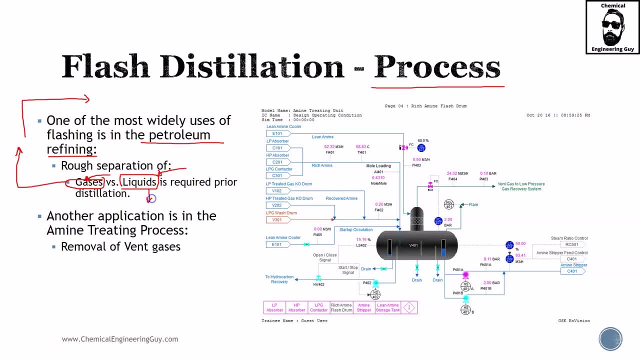 or more commonly, to a vent and burn it and you will get your liquid, which is stabilized. other type of applications may be amine treating processes, in which we use the removal of vent gases. so right here you can see here vent gas, because these materials are very- let's say not- volatile. they are non-condensable.